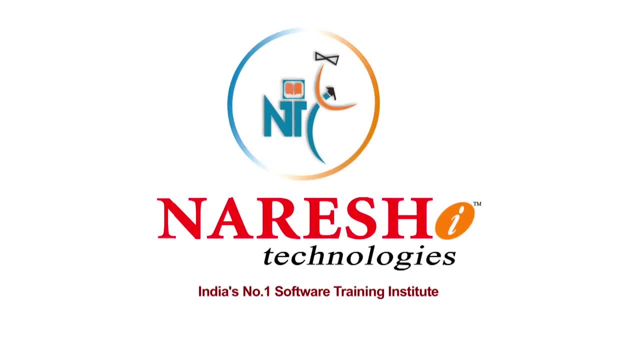 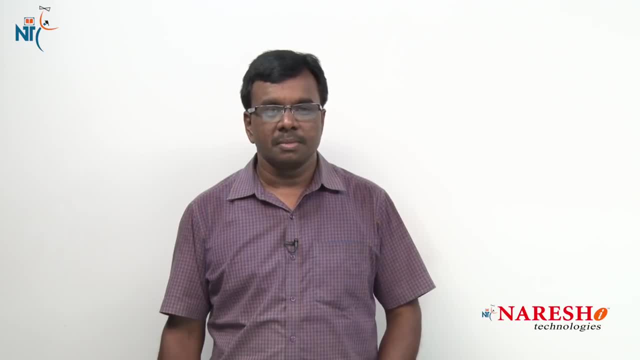 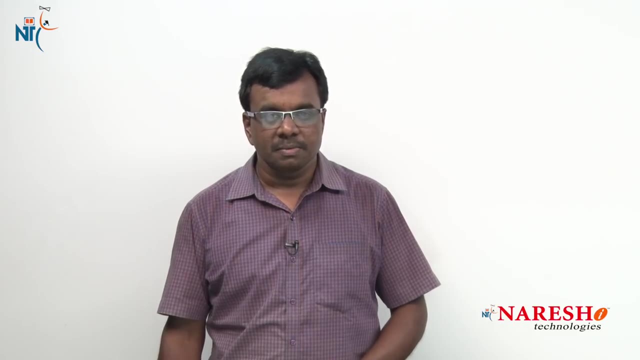 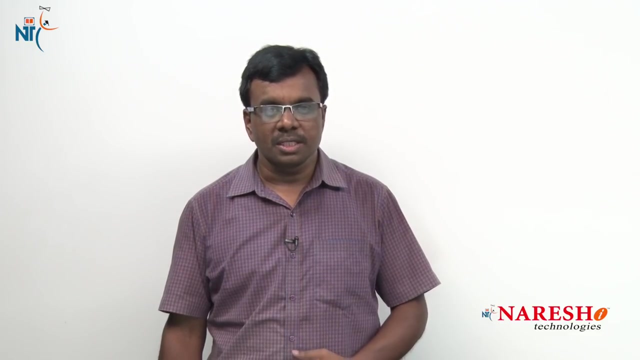 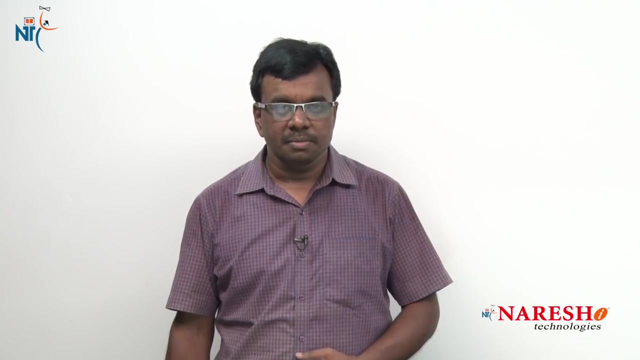 Hi, this is Vijay Kumar, So, having 10 plus years of experience in database technologies and data warehousing technologies, I got experience in database technologies like oracle, SQL, and having experience in database data warehouse technologies like Informatica and ODI, and. 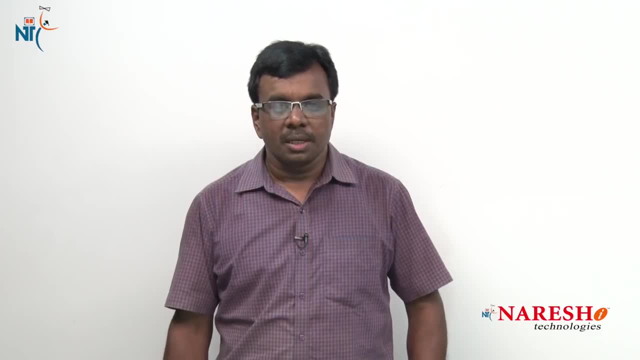 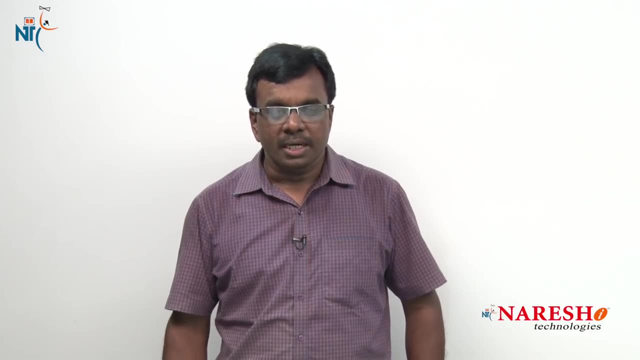 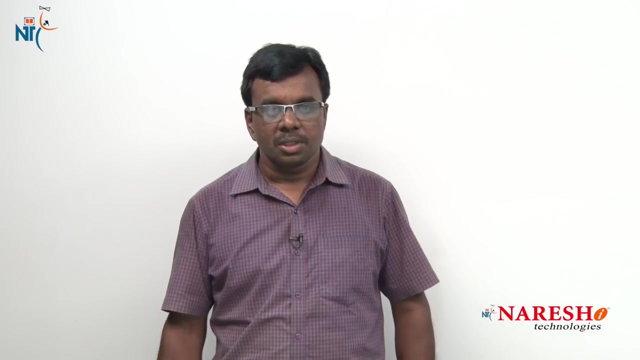 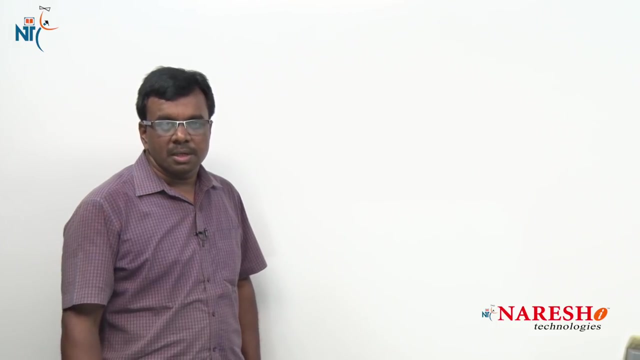 OBI. So in today's session, like we will see what is data warehouse, So I will give the introduction. So what is data warehouse and what is the need of data warehouse? So actually everyone knows a database. what is database? So almost all organizations maintains: 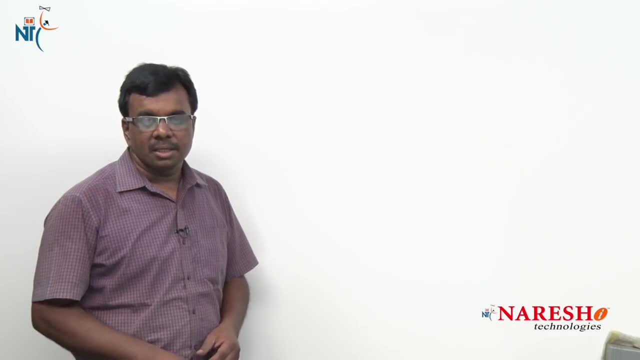 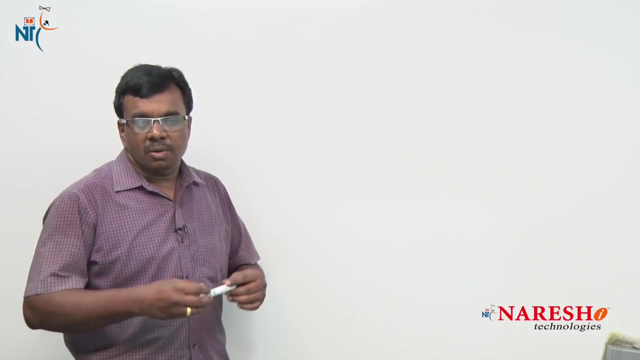 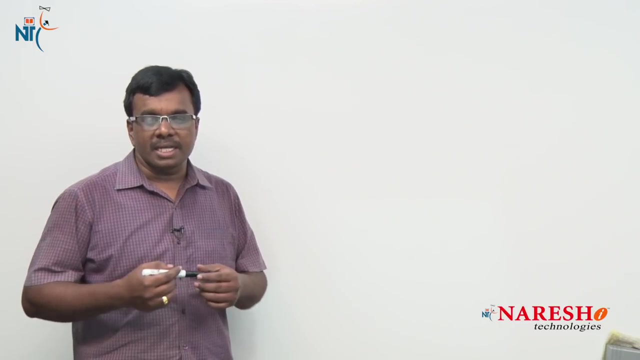 databases, like you take banks. banks maintains databases, and telecom companies maintains databases, and online shopping, So that those companies also maintains databases. So almost all, all companies maintains databases. what for? For storing day to day transactions. for storing day to day transactions like, for example, 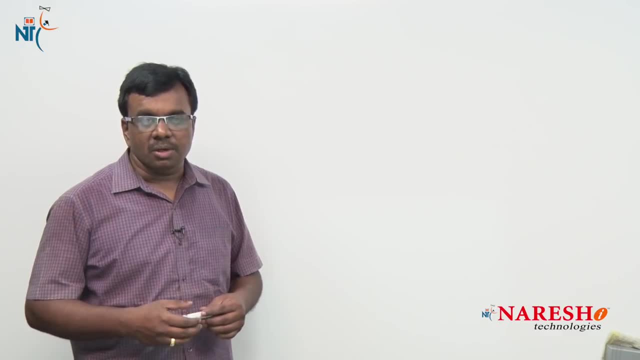 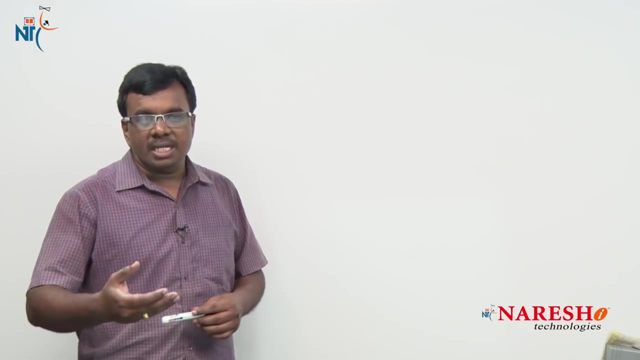 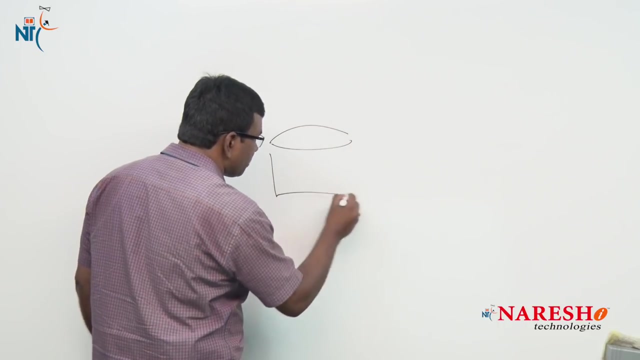 what are the day to day transactions in banks? So customers go to banks and customers deposit some amount, withdraw some amount and money transferred and all these details are stored in database. And what is this database is called? This database is called OEI. 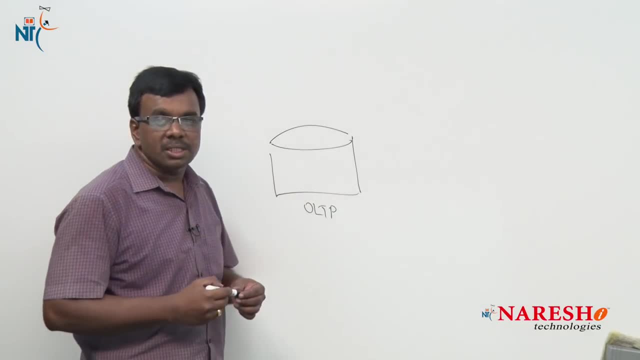 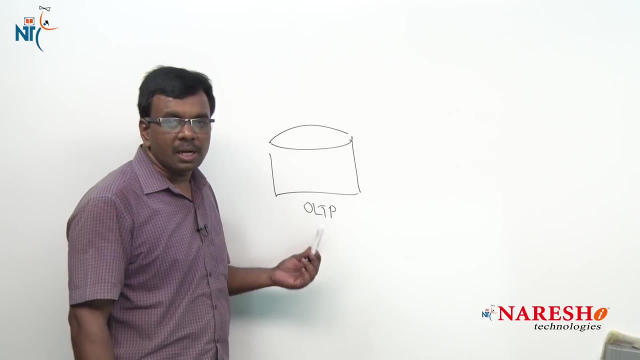 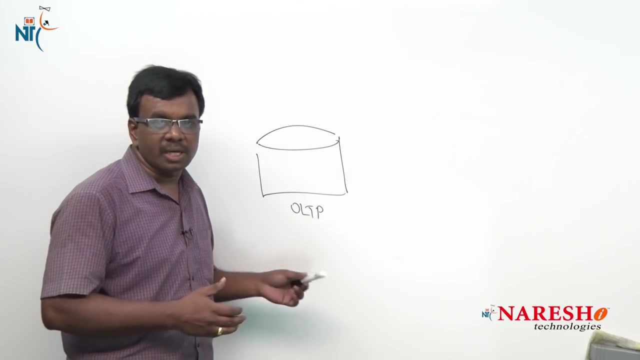 OLTP. Why? because So the purpose of this database is for storing day to day transactions. that is why it is called OLTP- online transaction processing. So every company needs this OLTP, like telecom companies maintains OLTP for storing customer's data and customer call. 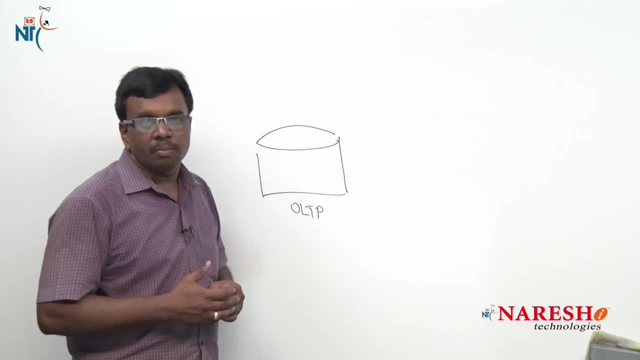 details. So online portals like, for example, flipkart maintains a database. So this database is called OEI And in the database they store what customer orders A customer go to flipkart and customer places order to buy products and all the transaction details are stored. 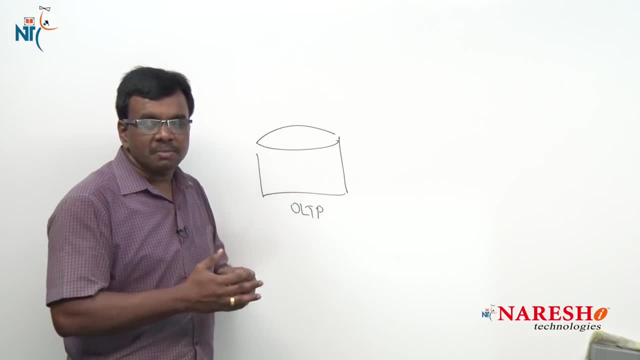 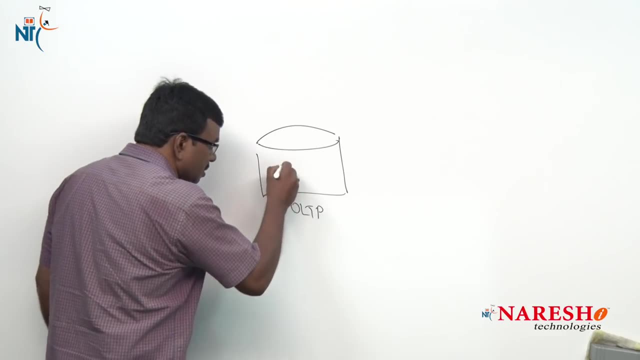 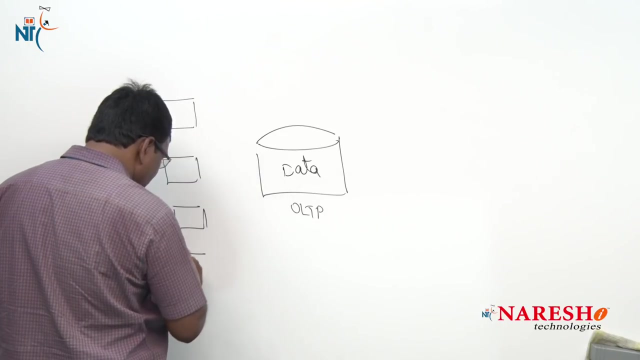 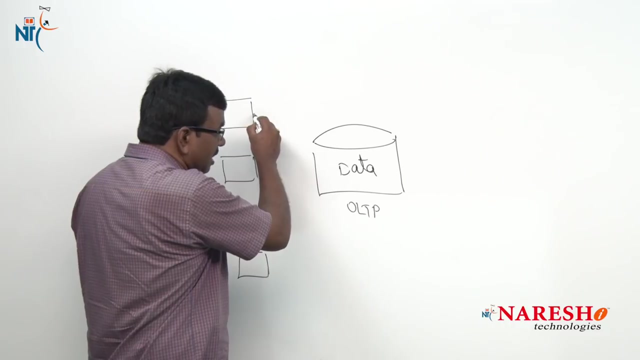 in database. So the purpose of this database is day to day operations, day to day transactions. So then, but what is the source for this data? The source for this data is applications. For example, you take banks, So there is application called transactions, So that application generates: 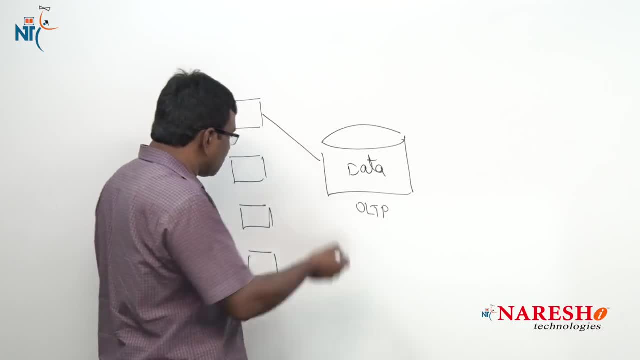 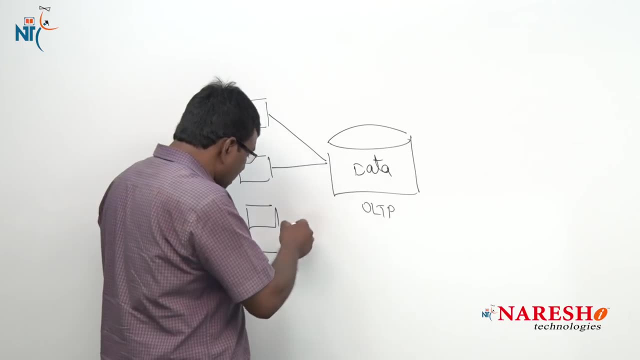 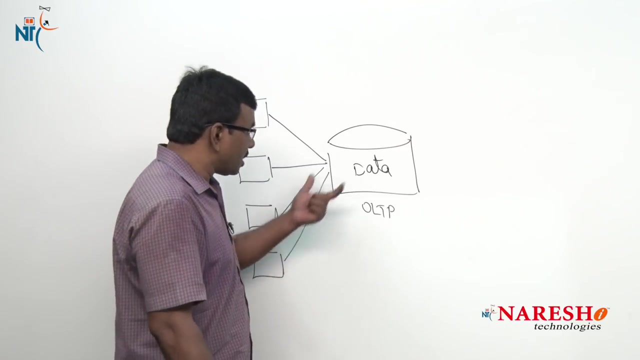 data, that data stored in OLTP. There is application called loans that generates data and stores in OLTP. So there is a call call loans. So there are different applications and this application generates data and the data stored in this OLTP database. So what is the source? 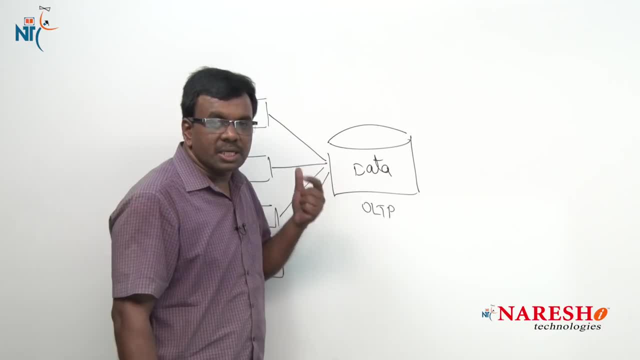 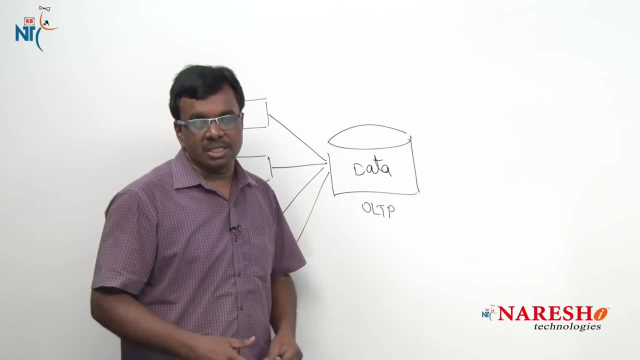 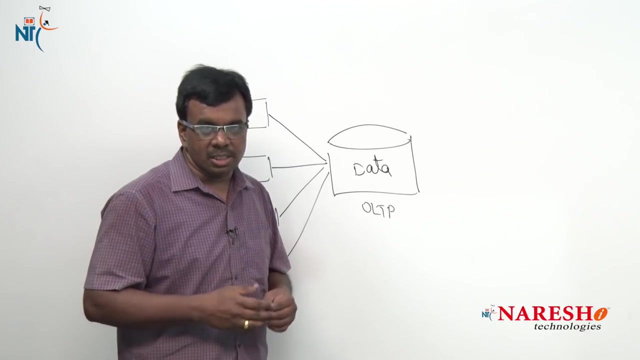 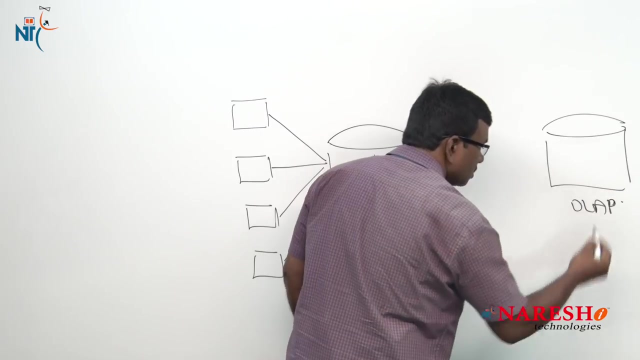 of this data. So applications: Application generates data and the data stored in OLTP. So, but nowadays, companies are using two databases Nowadays, so almost all organizations maintains two databases. So one database is OLTP and another database is OLAP. So what is OLAP? 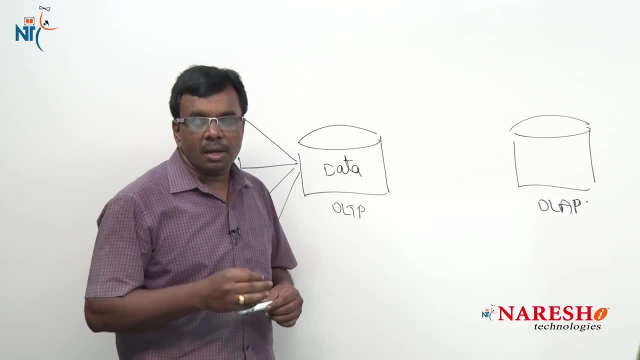 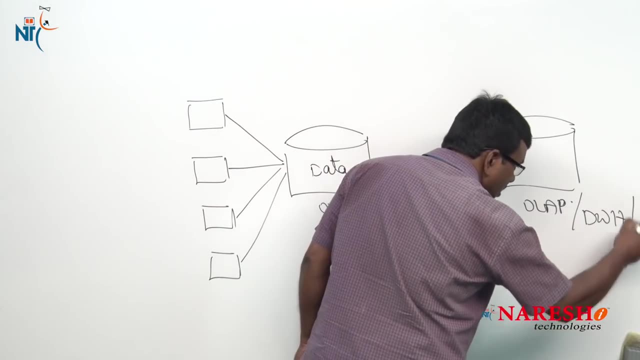 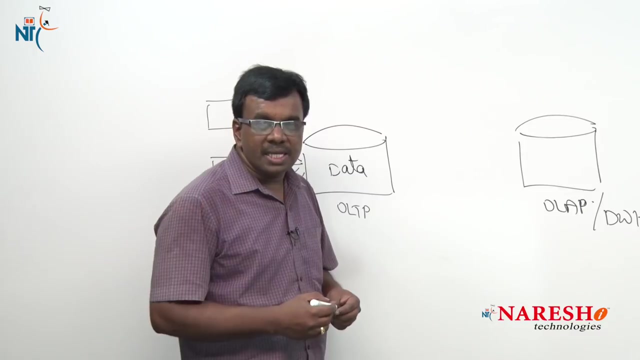 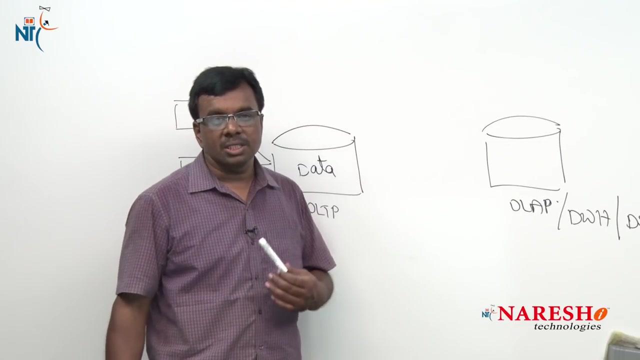 stands for OLAP, OLAP stands for OLAP stands for OLAP, OLAP. So DWH stands for data warehouse and DHS stands for decision support system. So nowadays almost all organizations maintains these two databases, OLTP and OLAP. So you know the. 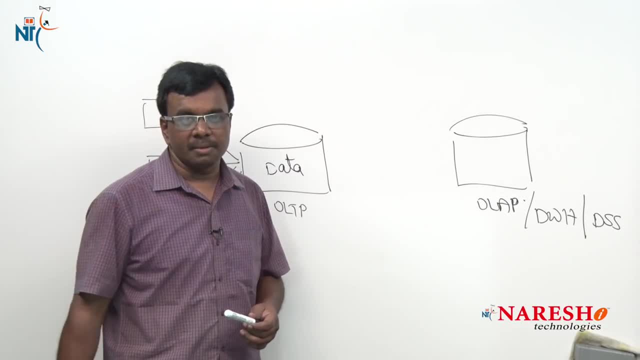 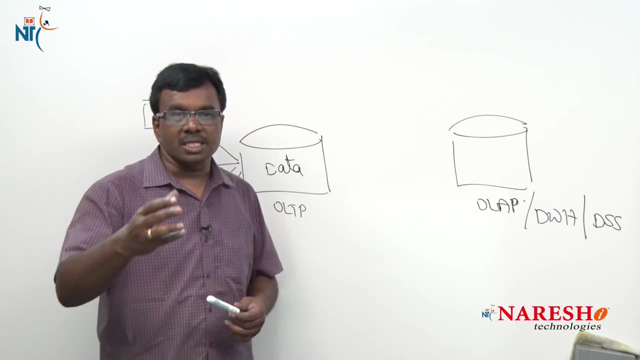 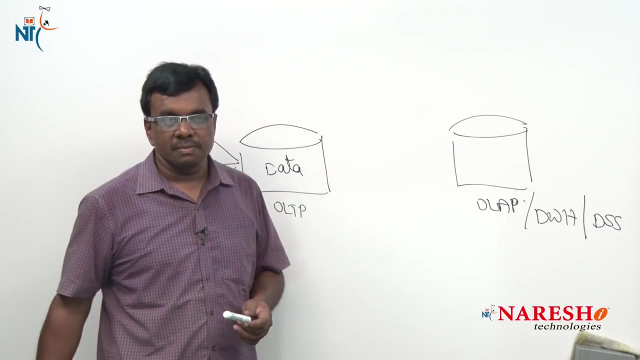 purpose of OLTP. So what is the purpose of OLAP? Why、 companies maintains OLAP. So companies maintains OLAP for analysis. So one database is for day to day operations, one database is for analysis and one database is for running the. 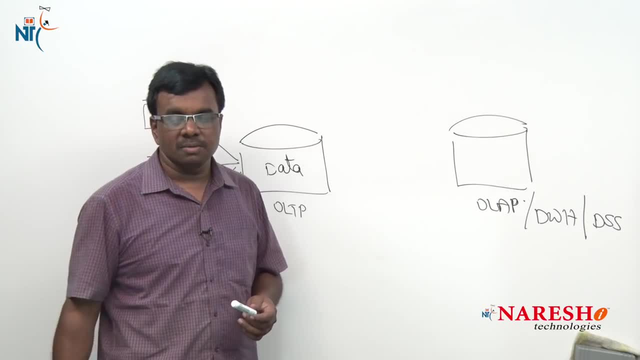 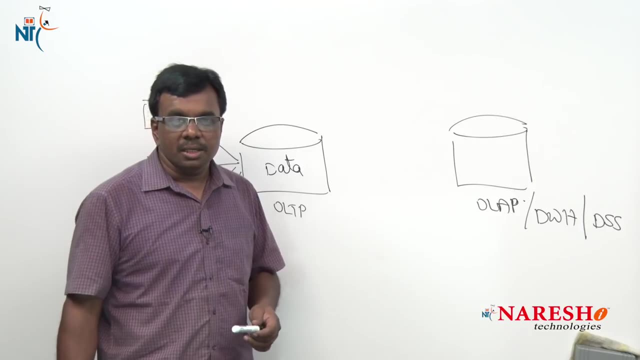 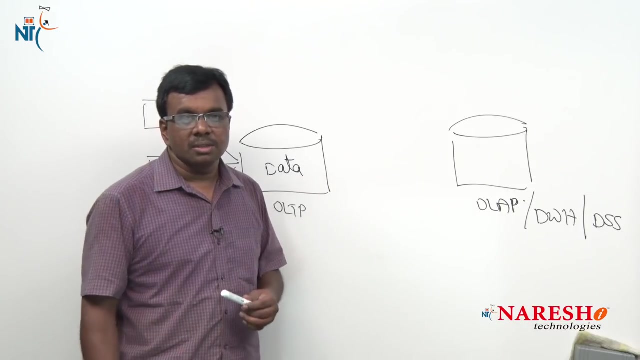 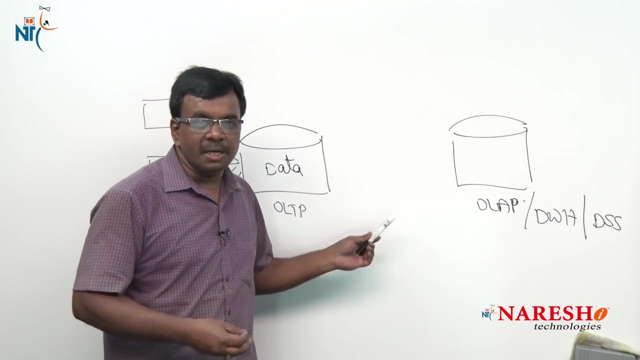 business and another database is to analyze the business. ok, One is for running the business, another is for to analyze the business. If company wants to run the business, they maintain OLTP. if the company wants to analyze the business, they need OLAP. The question is, why cannot we use OLTP for analysis? ok, why cannot we use OLTP database? 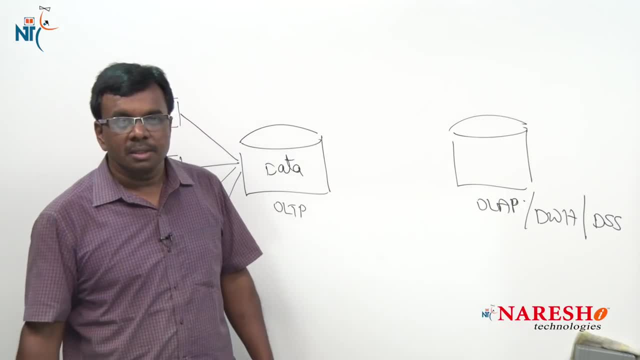 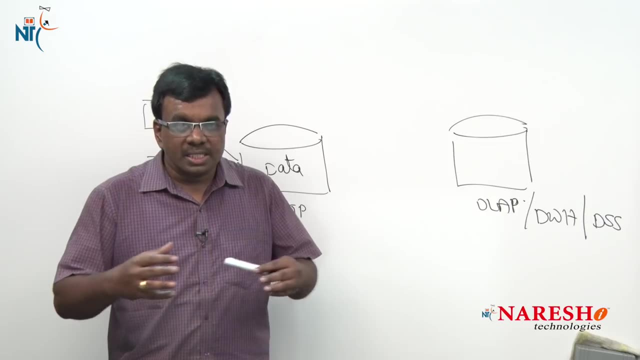 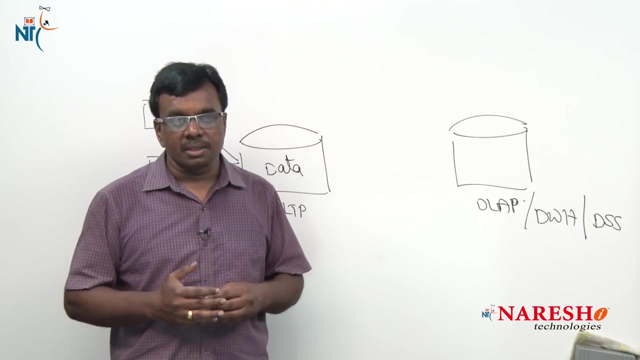 for analysis, why we need a separate database for analysis. So the reason is: for analysis what we need. we need history to analyze the data. we need history, Like suppose, here we is the best player in the cricket So I cannot decide it from current match, So if you know, 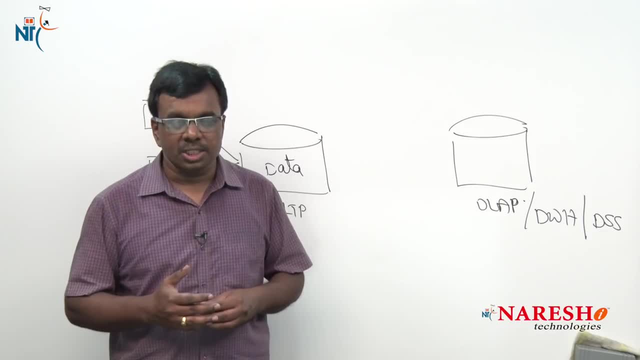 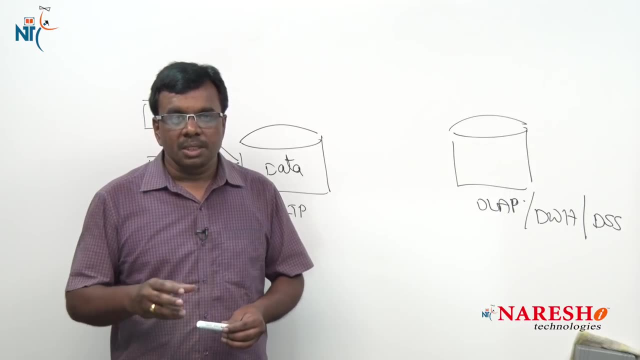 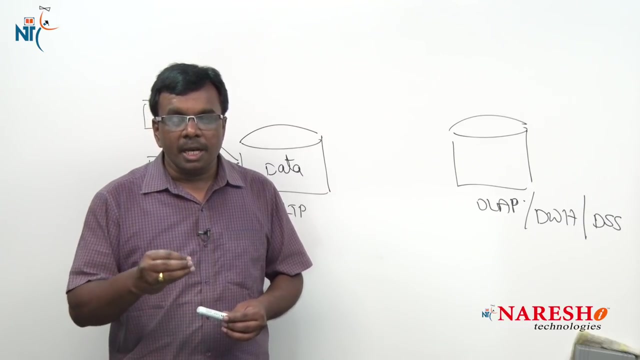 past 10 matches, then you can decide who is the best player in the cricket. So, similarly, in which state, like if you take countries, countries will be having states in which state population is increasing, in which state population is decreasing, in which state male population is increasing? in which state female population is decreasing? I want to find out. So, if you want to know this, then you need history, not 2017 years data. if you know past 5,, 10 years data, then you can able to decide. So, for analysis, what we need, we need history. 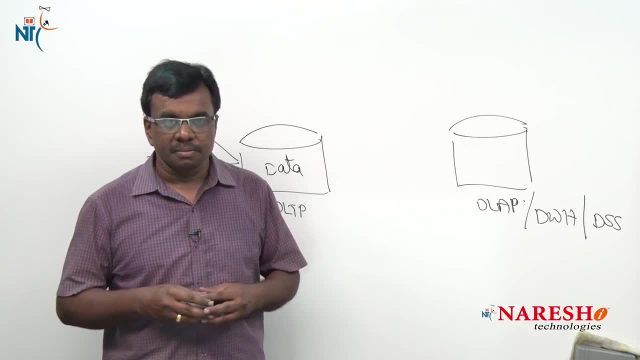 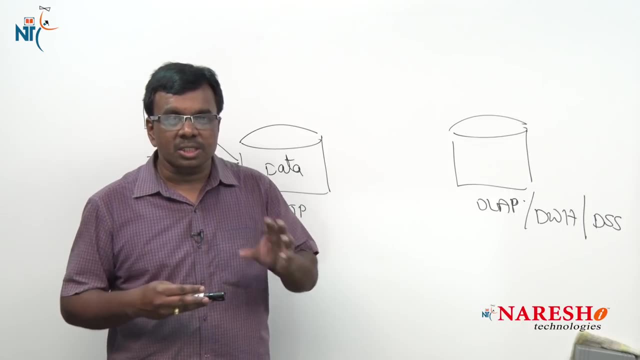 but what OLTP stores? OLTP stores current data, So it will not store historical data. only the current details of customers are stored in OLTP. why? because if you store history in OLTP, So the customer So the customer. So if you want to know this, then you need history. 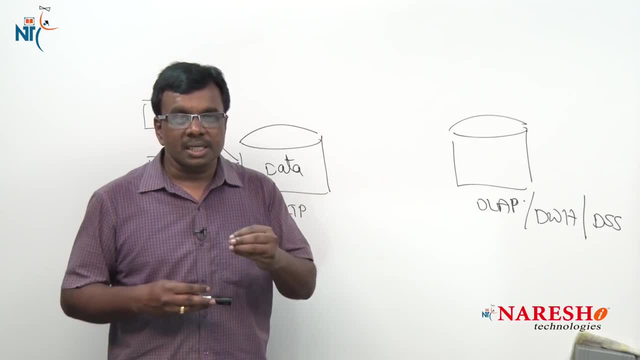 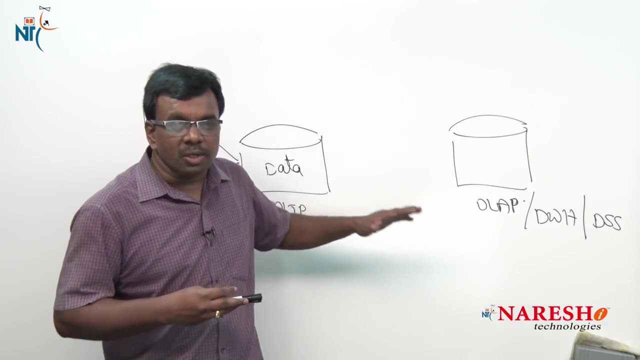 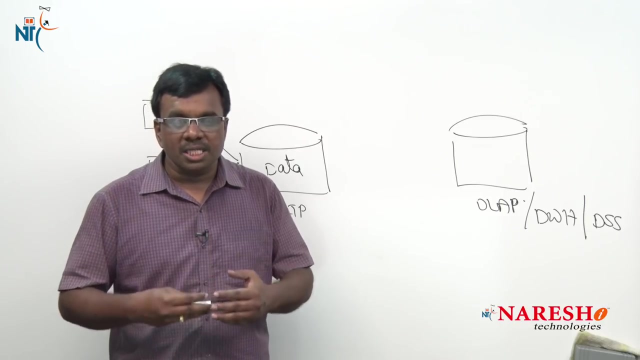 So the customer transactions gets affected and customer transactions takes half an hour time. So because of this, performance reasons, so OLTP, So it stores only current data. So when it stores current data we cannot use this database for analysis because for analysis 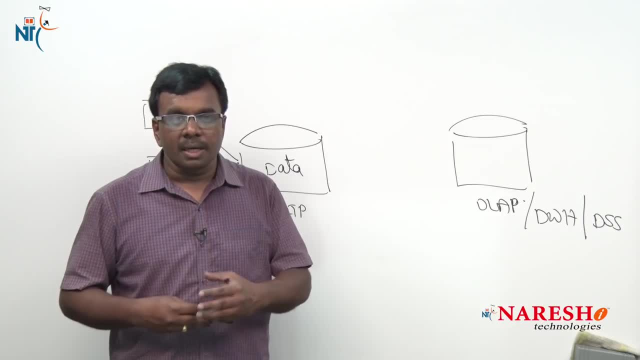 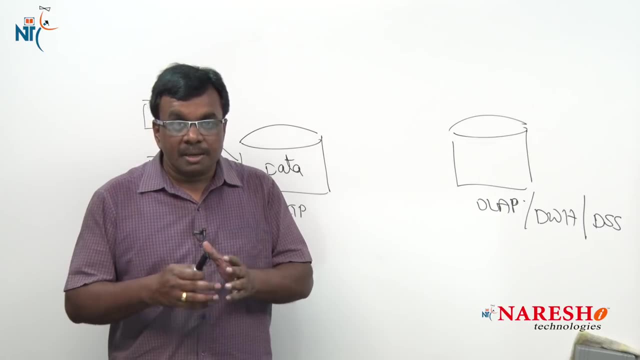 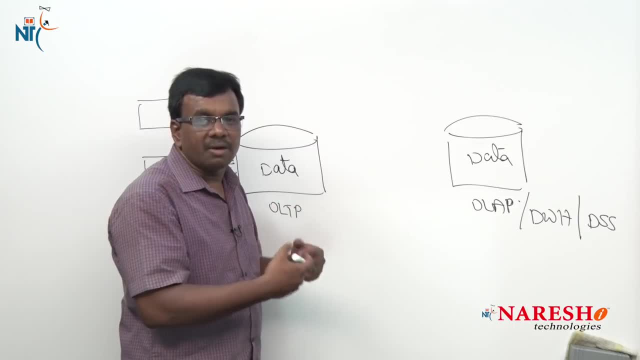 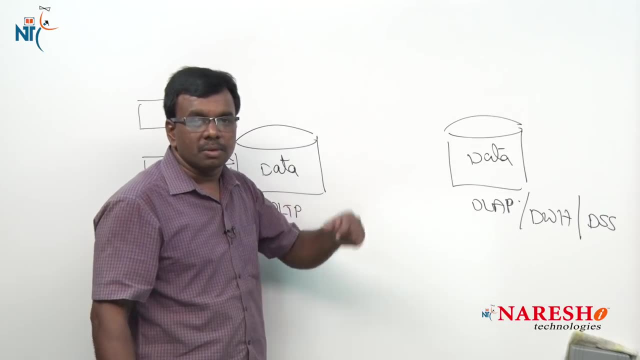 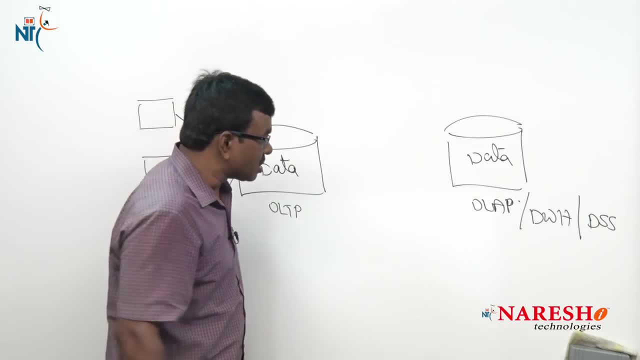 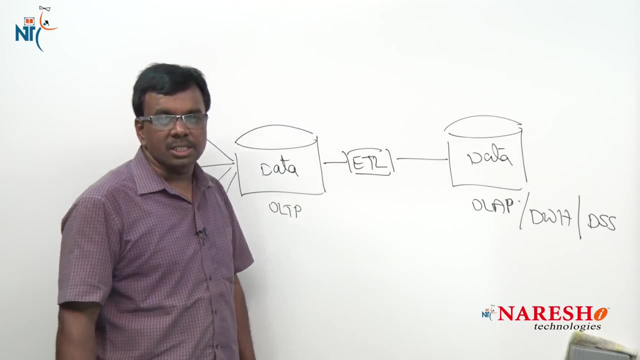 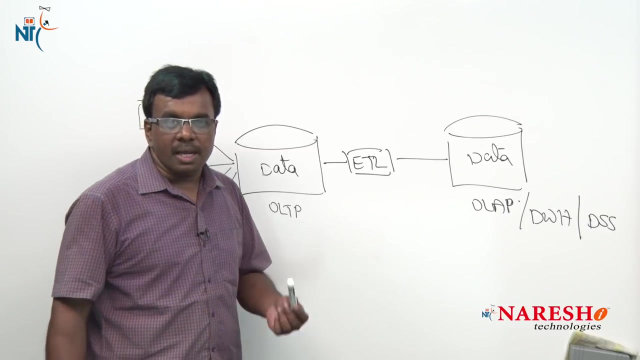 process of moving the data from OLTP to OLAP is called ETL process. The process of moving the data from OLTP to OLAP is called ETL process. What is ETL stands for? ETL stands for extract, T stands for transformation, L stands for loading, So extract the data from source. 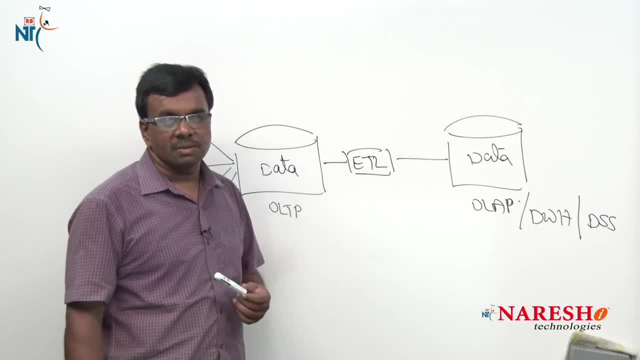 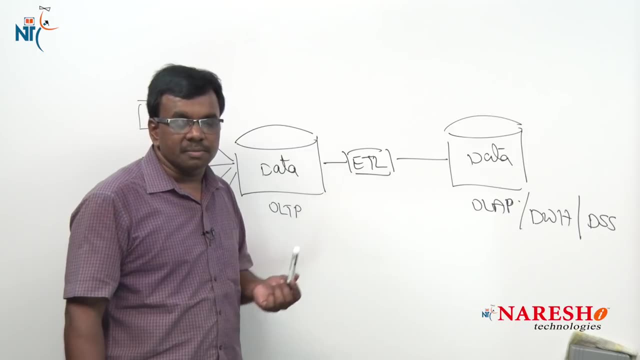 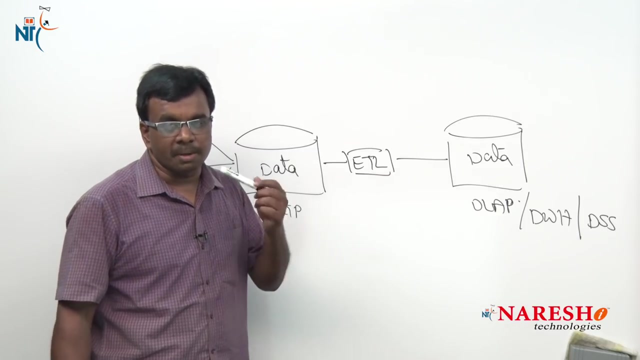 transform the data and load the data into database. So extract data from source that is, OLTP. transform the data, So extraction is simple, loading is simple. What is important here? Transformation is important, So you have to transform the data according to the. 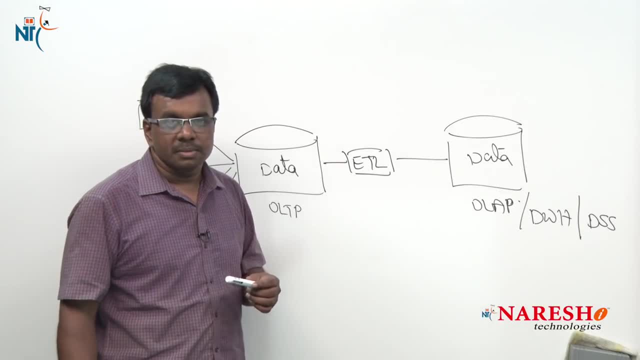 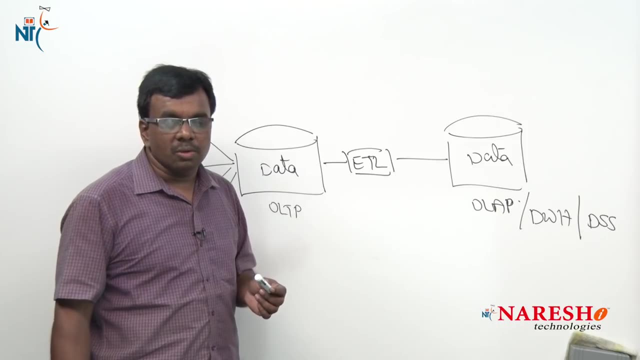 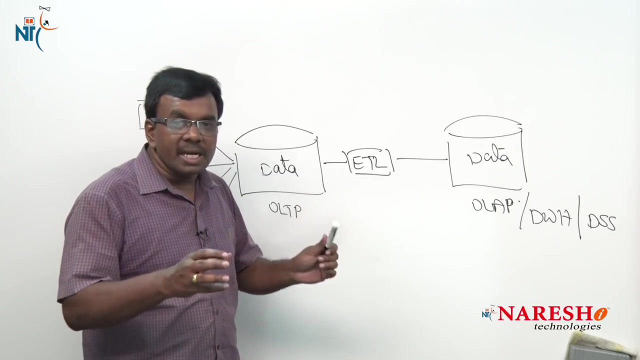 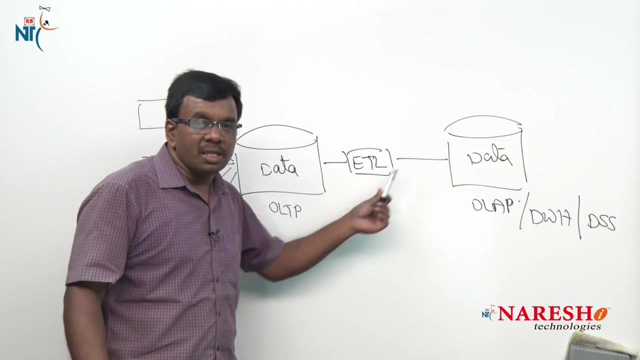 requirements of OLAP. you transform the data according to the requirements of analysis. So like suppose, for example here: So this OLTP stores like detailed data, but for I want to analyze the data for analysis, the data should be in summarized form. So before loading the data into OLAP, 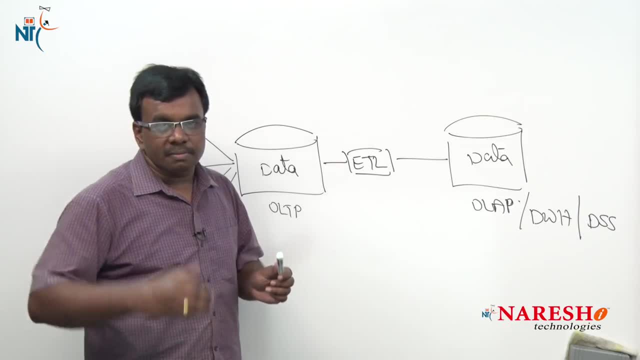 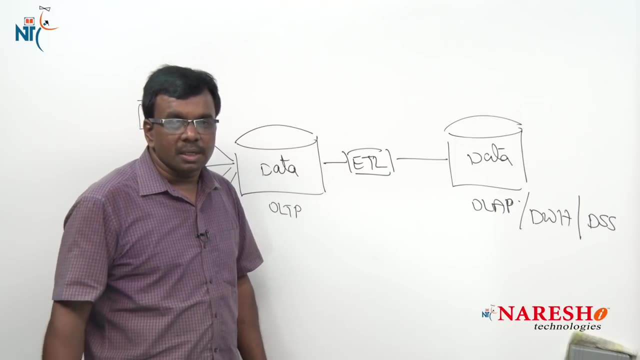 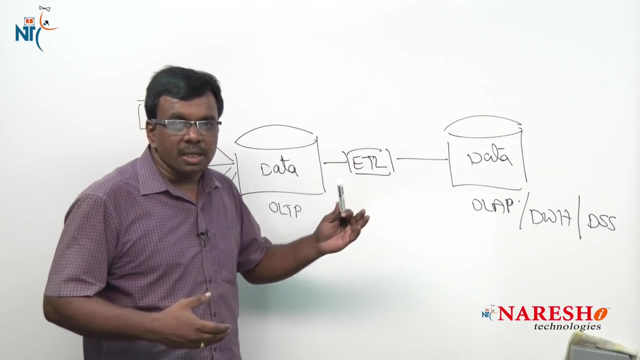 then first convert the data into summarized form, then load the data. So the one who wants to analyze so like he, wanted the dates to be in different format, like in OLTP system. date formats are something like MMDDYY, Suppose in analysis in OLAP system. I want date format. 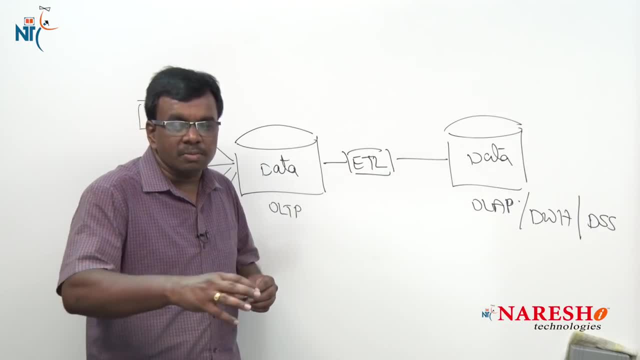 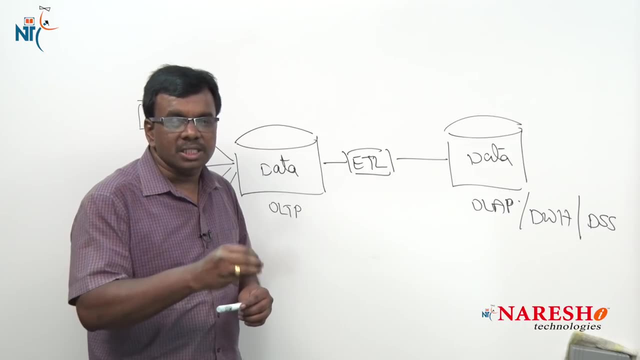 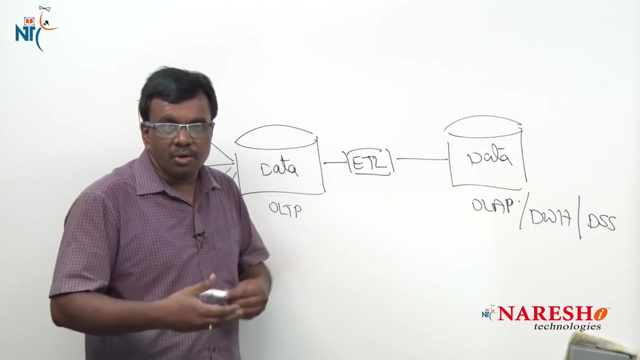 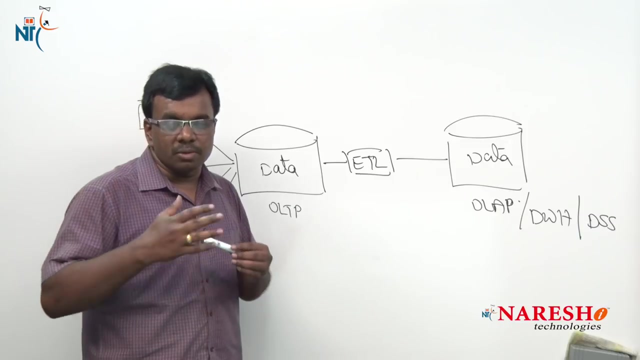 to be MMDDYY. So we need to transform the data. So extract, transform the data. next, finally, load the data into what data warehouse. but how this can be done? So do we? do we do this manually? No, So there are some tools. by using these tools we can do this. So 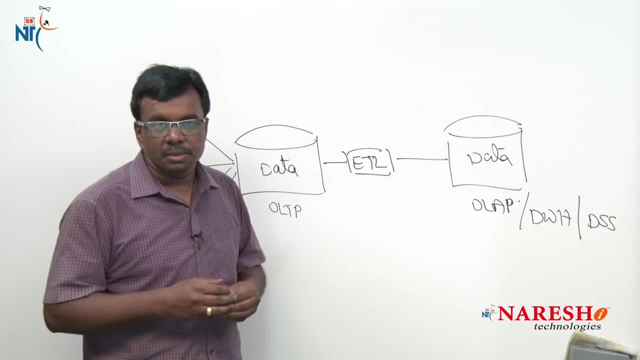 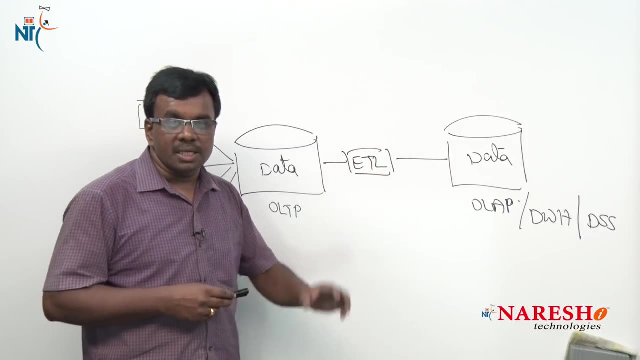 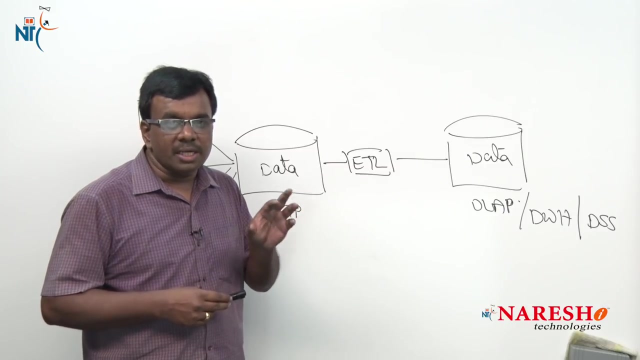 what are the tools? One tool is called Informatica, One tool is called Informatica, Using Informatica, so we can do this ETL process, and there is another tool called Talent. there is another tool called ODI, But ODI is somewhat different. So actually Informatica, Talendar, ETL, but what is ODI? 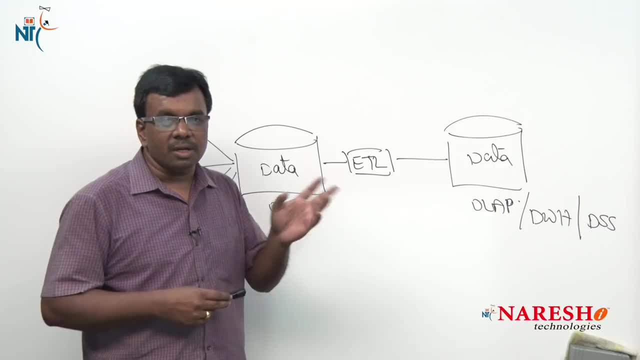 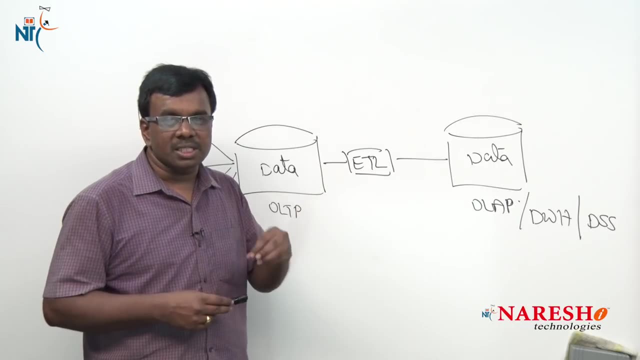 is ODI is ELT extract load transform. After loading the data, transform the data. So Informatica Talendar ETL extract transform load. but ODI is ELT extract load transform. 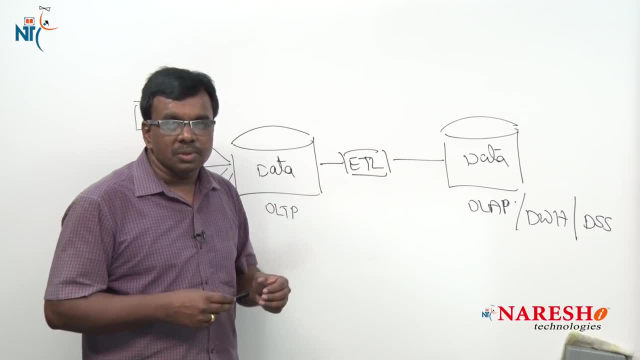 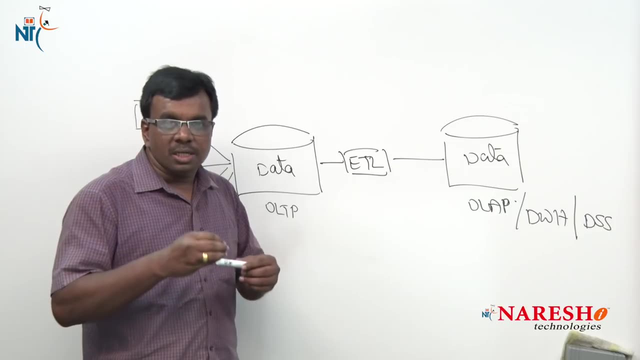 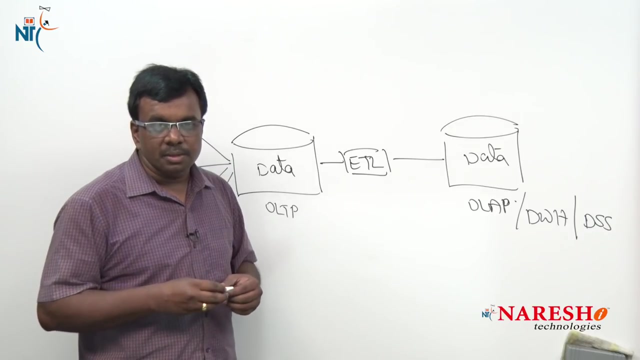 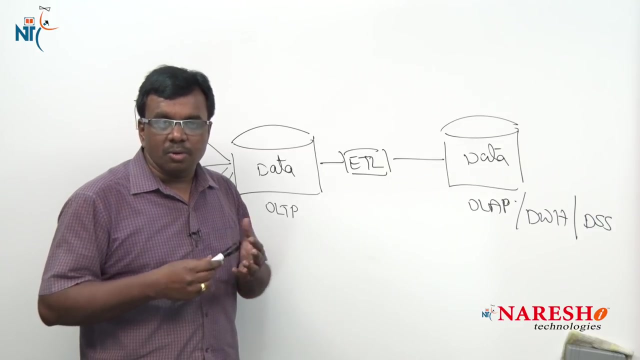 So after loading this data into data warehouse, you can analyze. but how to do the analysis To the to do the analysis? so we use. So there are some tools like tools like reporting tools are called BI tools, business intelligence tools. So what are the OLAP tools or BI tools or analytical tools like? example one is OBI. 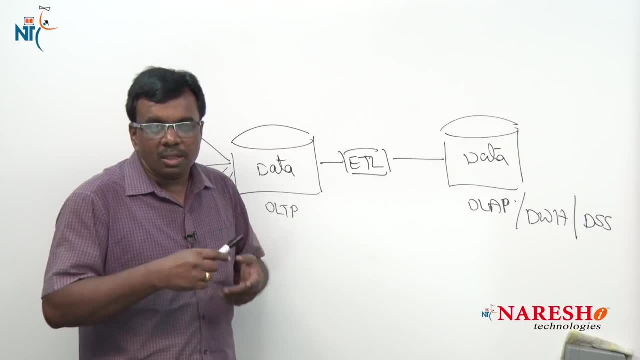 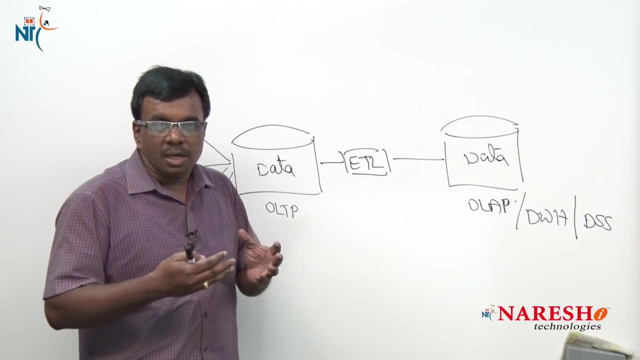 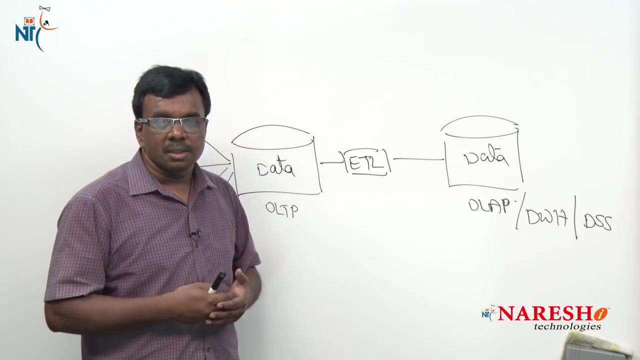 another one: click view, another one tableau. So all these tools are these tools are useful for reporting purpose? Once data loaded into data warehouse, I want to fetch the data, I want to analyze, So then. So then the tools used for analysis, like click view, OBI tabla, etcetera, microstrategy. So the 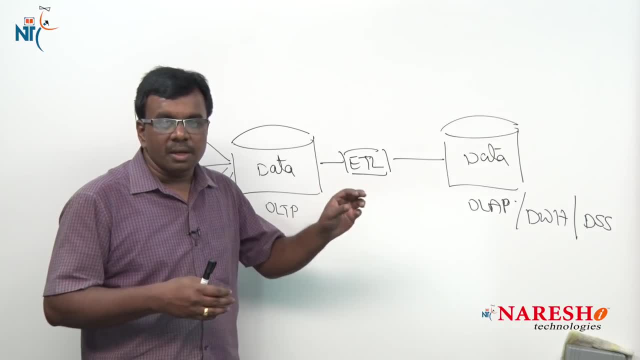 number of tools available. So this is the need of data warehouse. So thank you. Thank you for watching this video. For more videos, subscribe to Naresh IT.